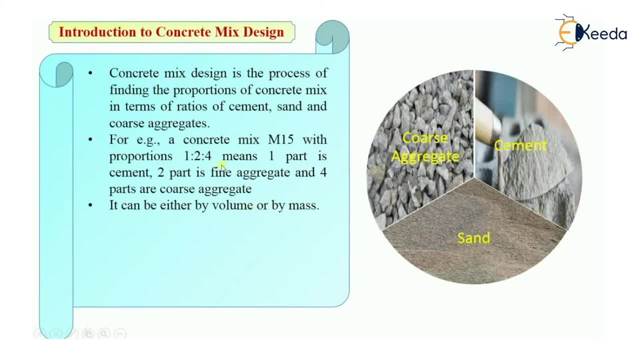 one. I am saying here one part is cement. that part may be taken in volume or in kg. For example, I am taking one kg of cement, then I will take two kg of fine aggregate and four kg of coarse aggregate. Or if you are taking in volume, say one CCC, one cubic centimeter or one-meter cube, for example. 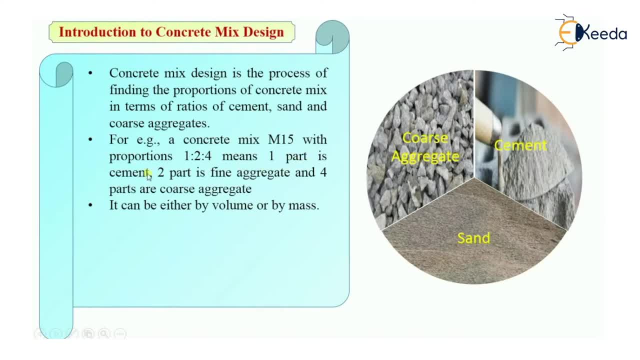 So I'm taking one meter cube of if. if I'm taking one meter cube of cement, I will take two meter cube of fine aggregate and four meter cube of coarse aggregate. So you can take it either by volume or by mass. It depends whether you are doing way bashing or volume. 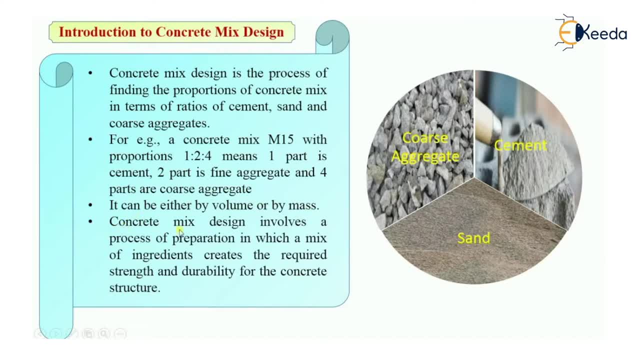 bashing And see concrete mix design involves a process of preparation in which a mix of ingredients will create� required КМ. will not be produced as mean or chrome guessing test or shifting to thediğence tractors for идеal shape of structure and age. designs involves a process of preparation in which a mix of ingredients will create required McHello or co felt coarse aggregates. So let's see the concrete mix design involves a process of preparation in which a mix of ingredients will create required cubeкуeling or coarse aggregates. 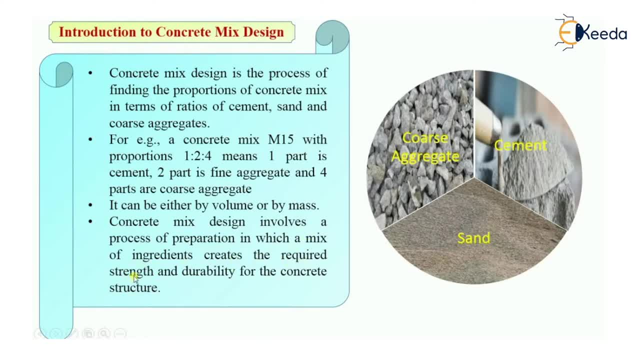 ingredients will create required strength, as we know that for m15 the required strength is 15 newton per mm square and we are achieving it by proportion of 1 is to 2 is to 4. so, similarly, concrete mix design will be a process in which we will achieve some required strength with. 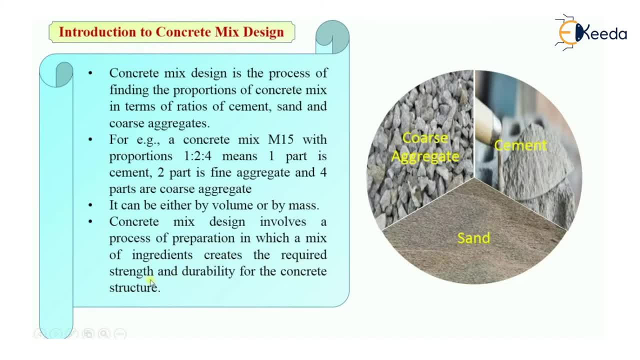 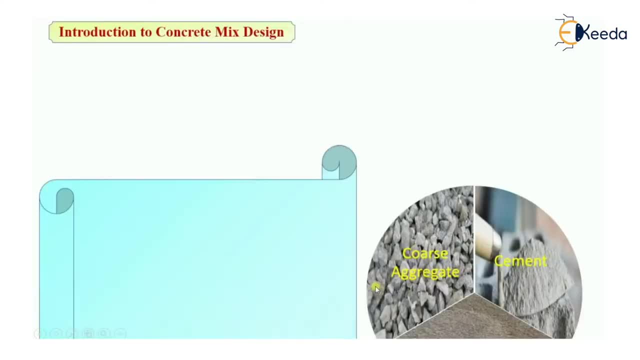 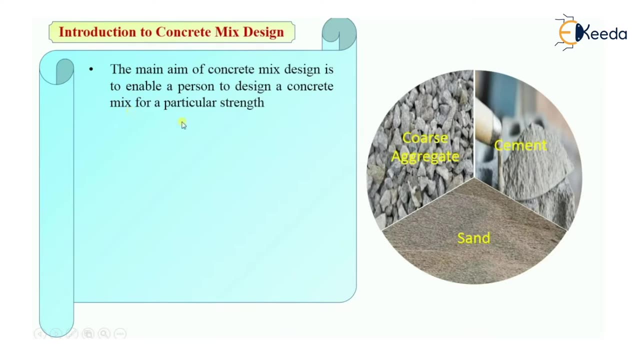 combination of ingredients or combination of various proportions of concrete mix and we can also achieve required strength as well as the durability of concrete structure. then the main aim of concrete mix is to enable a person to design a concrete mix for a particular strength. for example, if i want a for a particular structure, i want a compressive strength of say, 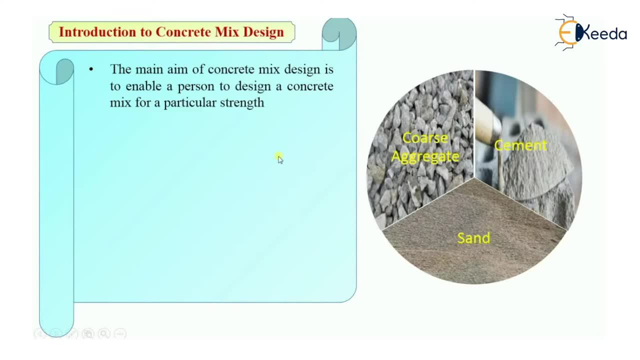 45 newton per mm square or 40 newton per mm square, so what? i will decide the proportions of cement, sand and coarse aggregate so that i will get maximum compressive strength at least 40 newton per mm square. that is my concrete structure and i will get maximum compressive strength at least 40 newton per mm square. 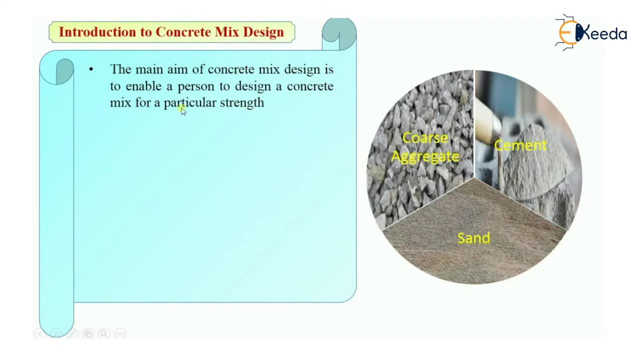 i want particular strength. for example, i am what i want- i want 40 newton per m square. that is my grade will be m40, so i want particular strength. so for that i will do the concrete mix design and see the structural engineer at the time of designing a structure will stipulate certain 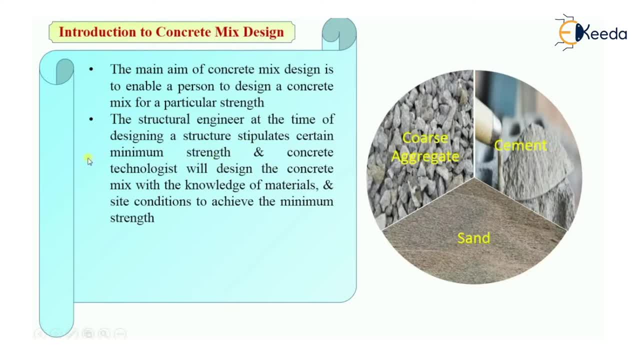 minimum strength. for example, in structural drawing, the structural engineer will mention in the node that this concrete structure should have minimum compressive strength. of this. this, for example, m20 should be used, m30 should be used. so he he will stipulate certain minimum strength and concrete. 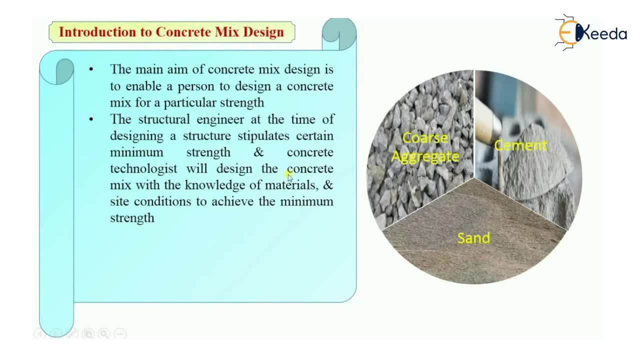 technologist will design that concrete strength or concrete mix, with the knowledge of, say, materials, site conditions, and he will design in a such a way that that we can achieve that minimum strength which which has stipulated by the structural engineer. so structural engineer will stipulate the minimum strength and concrete technologist will design that strength mix and every. 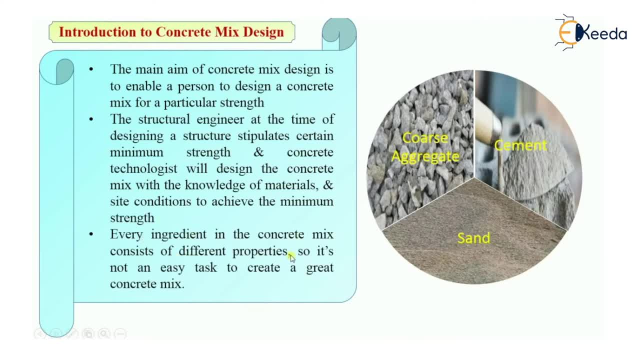 ingredient in the concrete mix will consist of different properties. for example, cement will have some different properties, sand will have some different properties, coarse aggregate will have different property. each and every ingredient of concrete mix will have different property. so it is not very easy task to create a great concrete mix. we will require some trial batches, trial mixes. 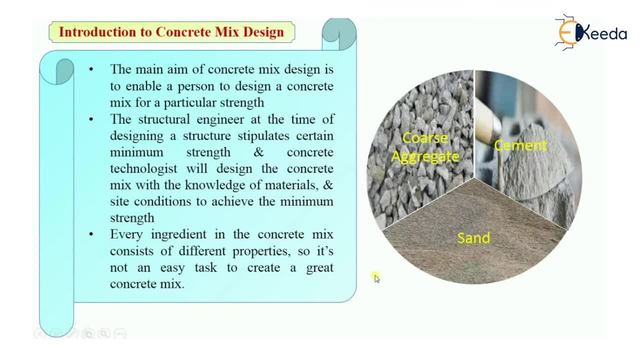 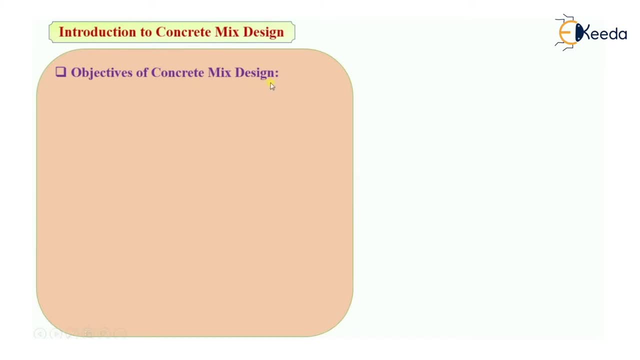 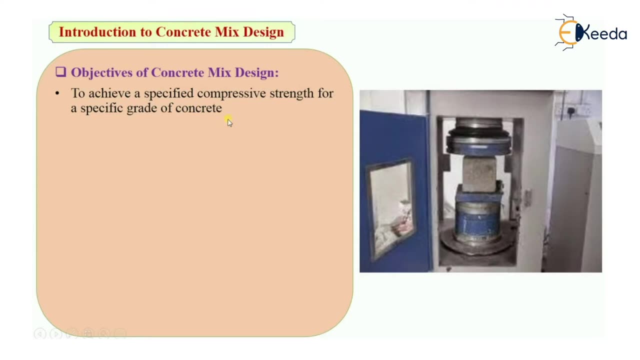 so that we can achieve the final concrete strength which is required strength. now let's see what are the objectives of concrete mix design first. the first objective of it is to achieve a specified compressive strength for a specific grade of concrete, as i told you before that. for example, 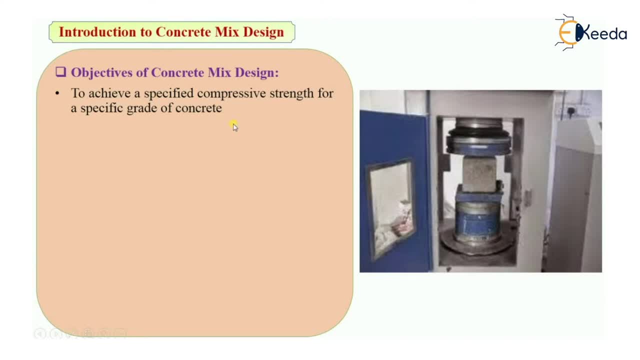 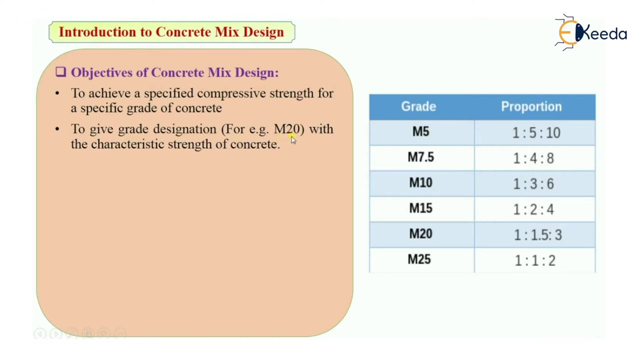 i want m40 grade of concrete, so my specified compressive strength will be 40 newton per m square. so to achieve some specified compressive strength for a specific grade of concrete, we can do the concrete mix design then to give grade designation, for example m20. m20 is nothing but a grade designation, where m stands for mix and 20 stands for. 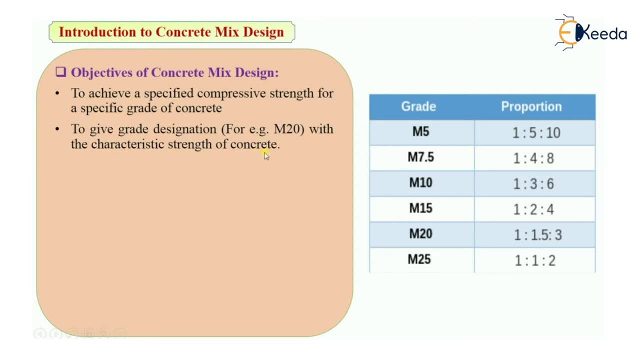 compressive strength of concrete in newton per mm square in 28 days. so to give greater designation with characteristic strength of concrete, we can design the. we can do the concrete mix design. as you can see in the table here, these are nothing but different grades of concrete which are used and on the right side its proportion is given, for example for m10. 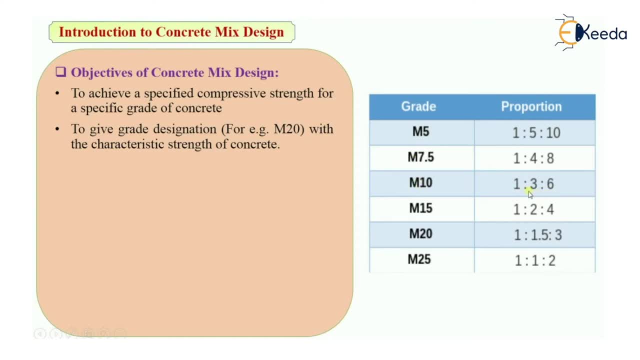 the proportion will be: 1 is to 3 is to 6. one part of cement, three part of sand or fine aggregate and six parts will be of coarse aggregate. so for m5 it is one, one, five, ten, that is, one is to five to ten.